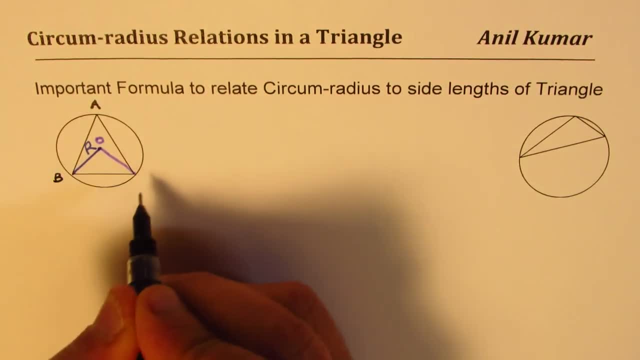 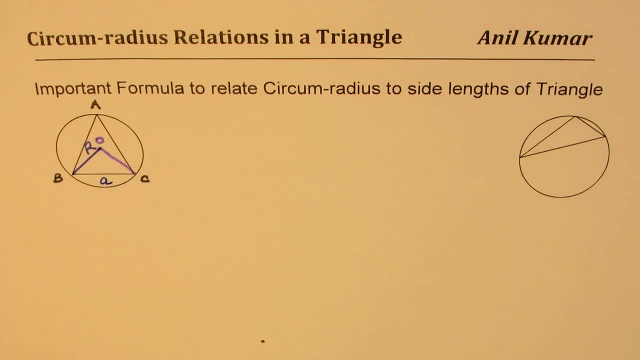 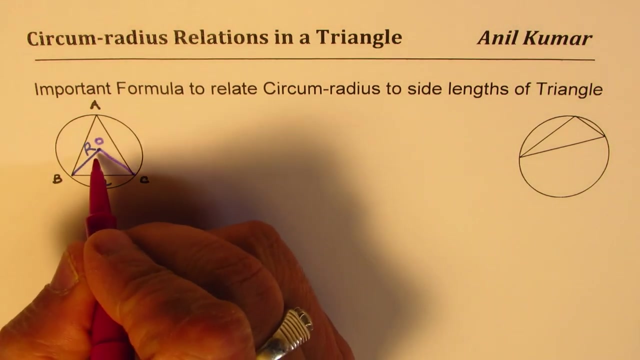 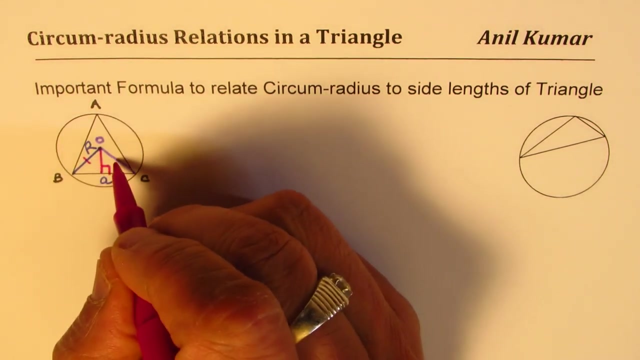 ABC. So side opposite to A will refer to as lower case a right. Now let us say that I drop a perpendicular from the center to BC. Now, since these are the two radii of a circle, they are same. 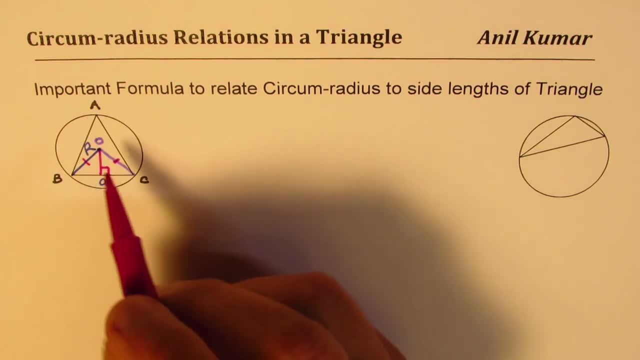 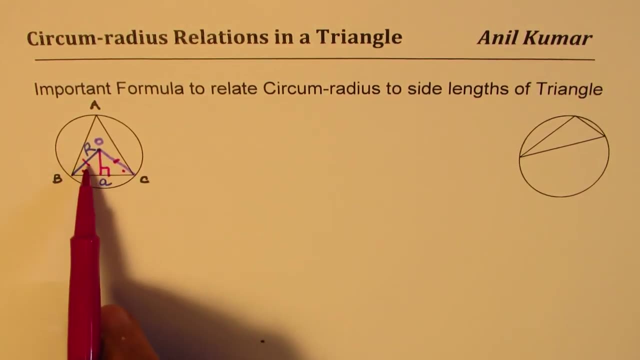 correct? And therefore we will have the same angles also here, correct? And we have 90 degrees. So these are common side, So these are actually congruent triangles, correct? So in that case, the length here. let us call this point as a D, right? So in that case we know BD. 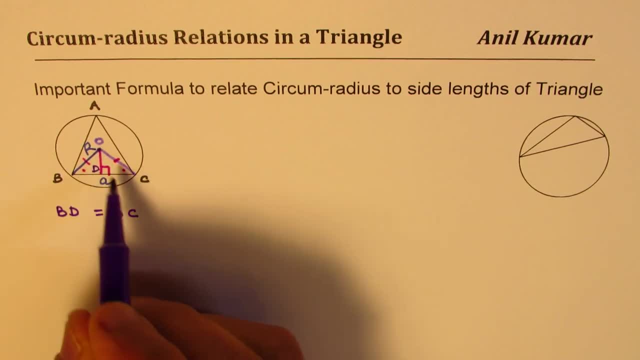 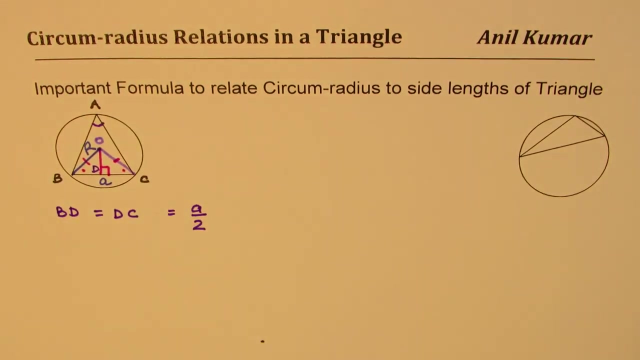 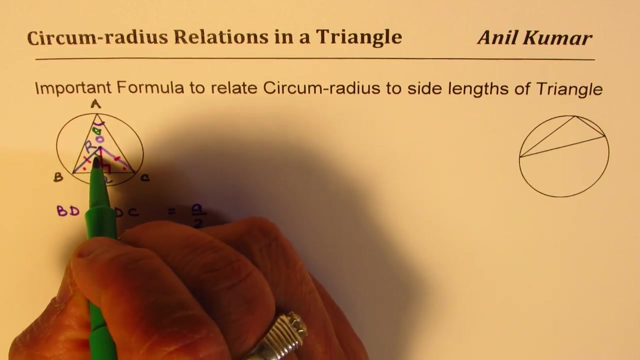 will be equals to DC and both will be equal to half of A. Now let us say the angle here is theta. Let me use a different color here. If this angle is theta, the total angle at the center will be 2 theta. So the smaller angle will be also theta, correct? 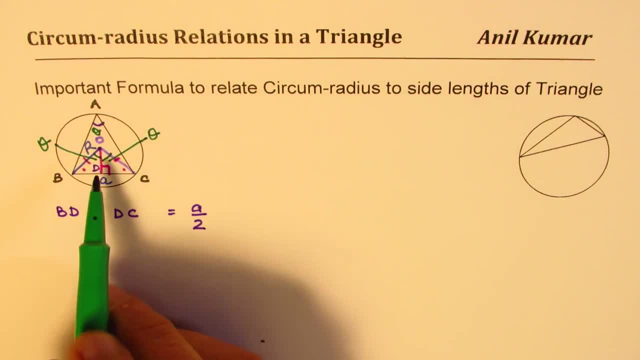 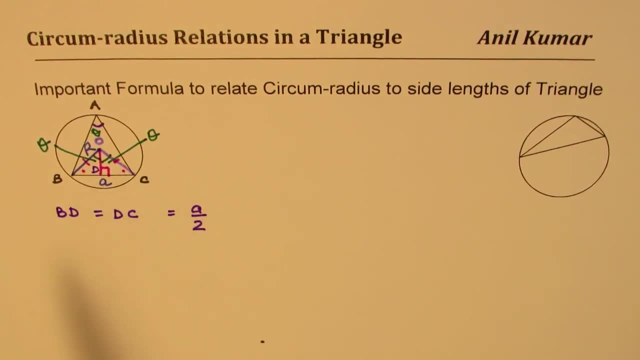 These two will also be theta each, because the center angle will be twice that angle right. So now we have a right triangle. So if you look into the triangle which is BDO, in this particular triangle what is sine theta equals to Well, sine theta is opposite side over hypotenuse. The opposite side is BD, and 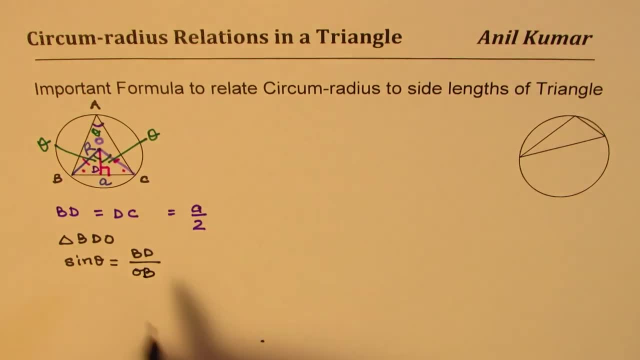 the hypotenuse is OB, So from here you can see that sine theta is basically equal to B to D, is half times A, and OB is our capital R Right, the circum radius right. So from here we can see that deductions between circum 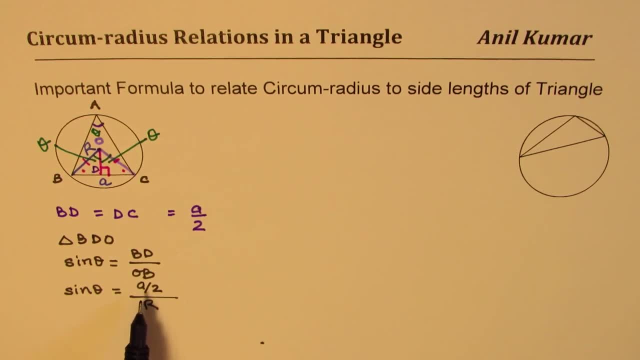 radius and the side length, correct. So if I cross multiply I get radius is equal to A by 2 sine theta, correct? So that becomes a relation between the radius this side and the angle above it. it like a sin law, right? So if you want to relate it to sin law situation you can actually 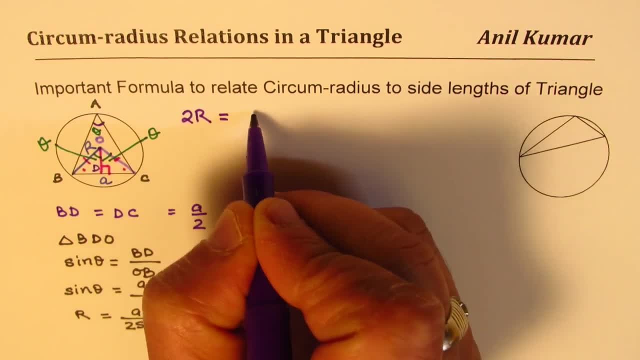 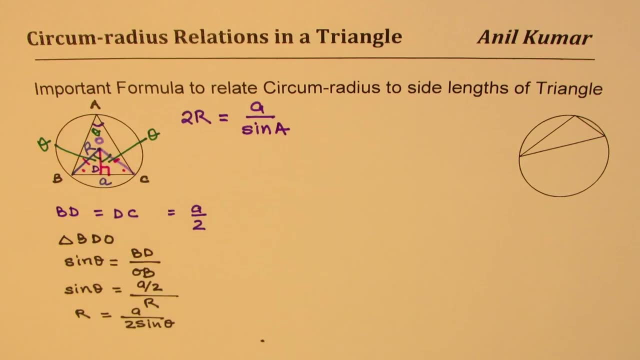 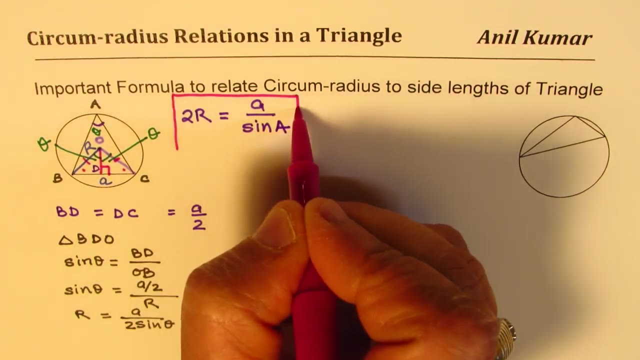 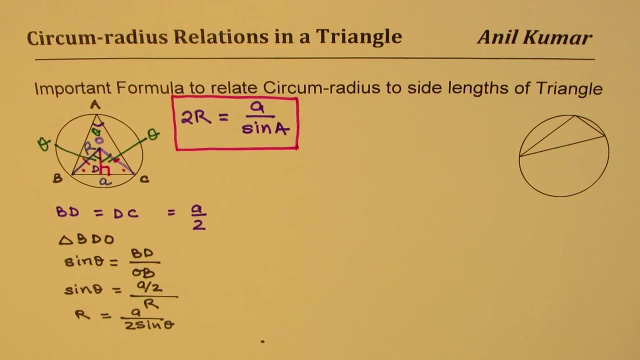 write this formula as: 2 r equals to a over sin a, because this angle, theta, is actually the angle a right. So that is how we can actually relate circum radius with angles and sides of a triangle. that is a very important formula. Now let 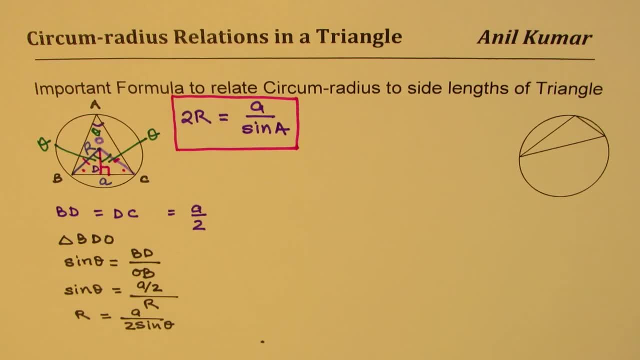 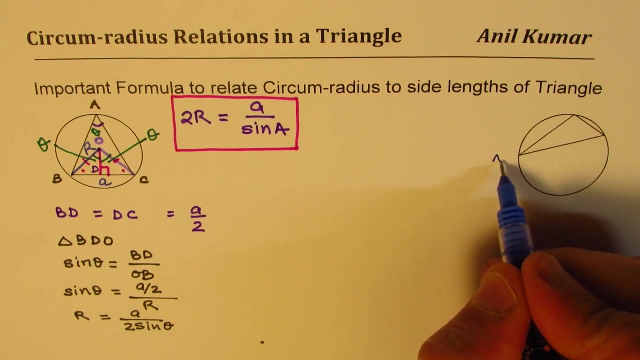 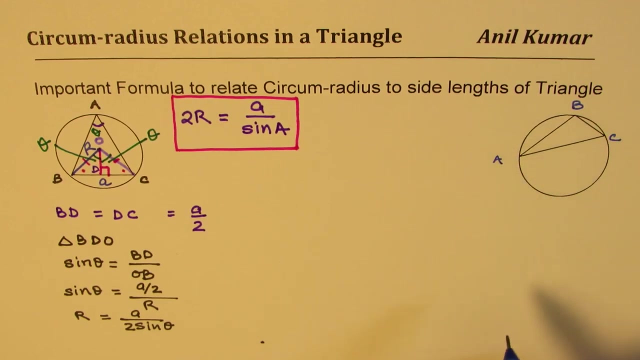 us also derive another formula where we will relate the side lengths with the circum radius. So for that I have a triangle here and we will take this triangle as, let us say, triangle a, b, c, any triangle Which is circumscribed with this particular circle. Now let us join point b with the 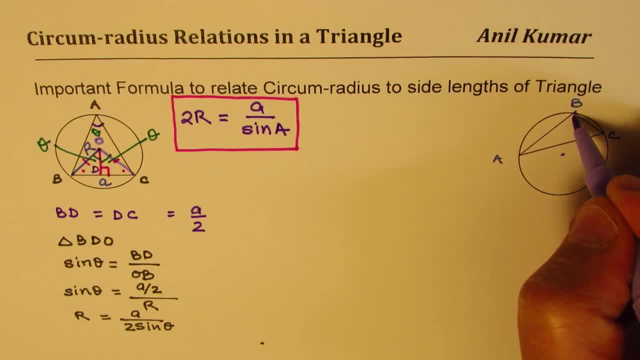 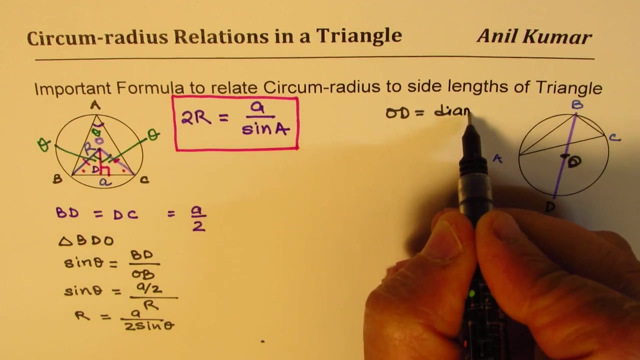 centre of the circle right. Let us say this is the circle centre. then that becomes the diameter right. Let us call this point as point d. So in that case this length b to b circum is 0. Let me think The circum centre will put o right, put the d here. So. 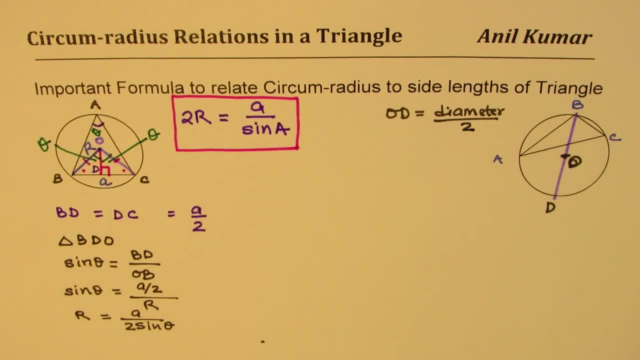 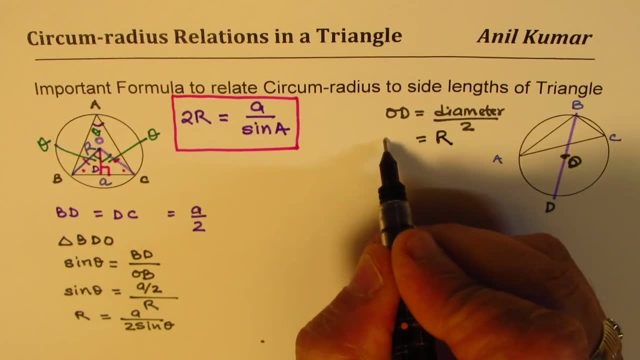 in that case what we have here is od is the diameter right, half the diameter, because b to d is the diameter. I write od half of the diameter. So which is the radius r for us? we will call this as a radius of r, and these two, these are the di am gate right we have. the radius r, whatever deeds are present between the two of them. Now, when we we have a point, this portion, we white forward. So would not it judge the red part? where does it reduce the diameter? r will be the radius of r to c, or the right position. Now we have, we done, and 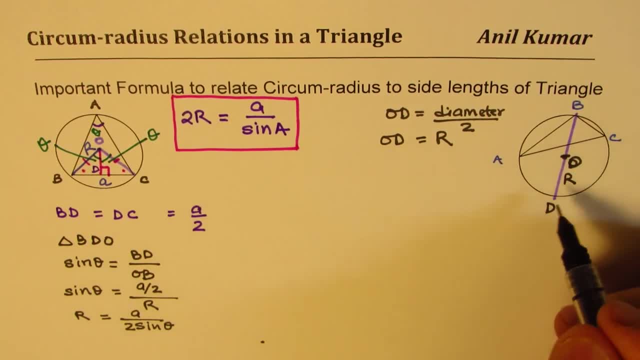 the circum radius. now we need to find this radius with respect to sides ABC of a triangle. now, in this particular triangle, let me drop a perpendicular from B to base AC. let this be the perpendicular. this side be this point be e, and let us say that so that becomes a perpendicular. now, if I join points A, 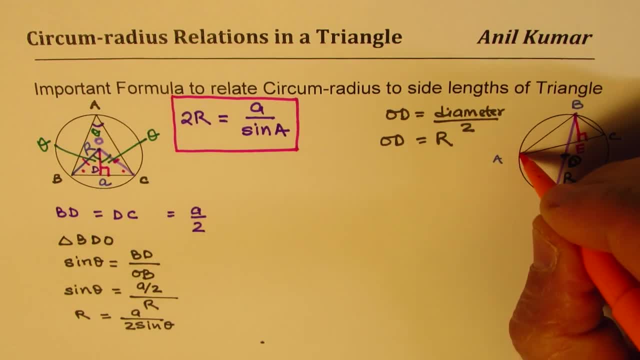 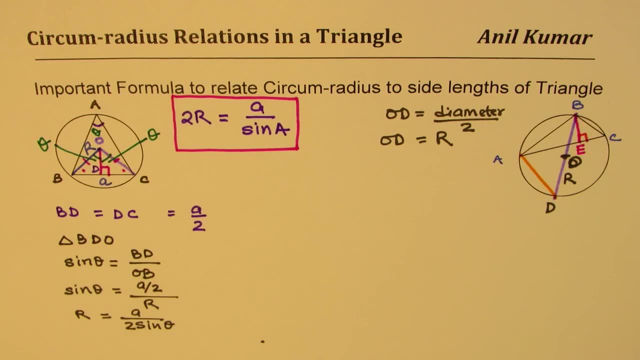 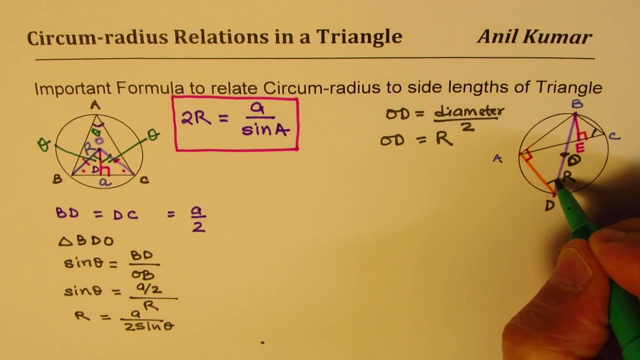 and D. in that case, that is a semicircle. so in semicircle we'll have a semicircle. so in semicircle, we'll have a right triangle. so that becomes a right triangle. perfect. now we also see that these two angles, they should be equal, reason being that both these angles are. 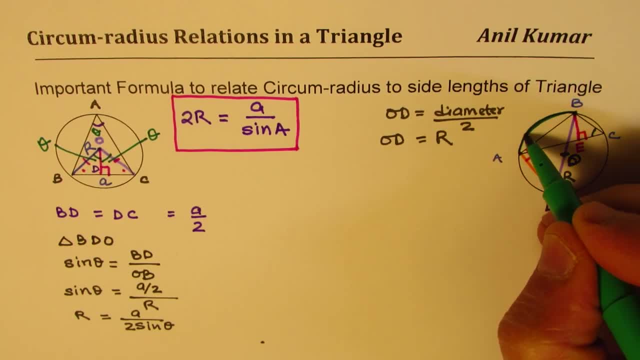 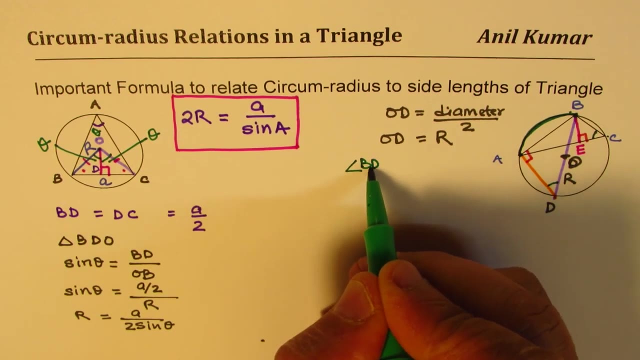 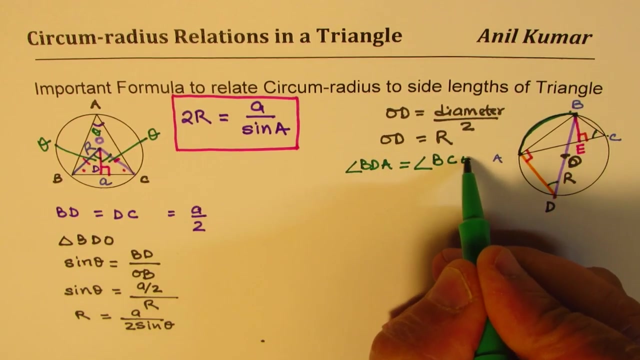 on the same arc, arc AB right. so this angle, angle BDA and angle BCA- both are on the same angle. so these two angles are on the same angle. so these two angles are. so we have that angle BDA is equal to angle BCE and there is 90 degrees. so 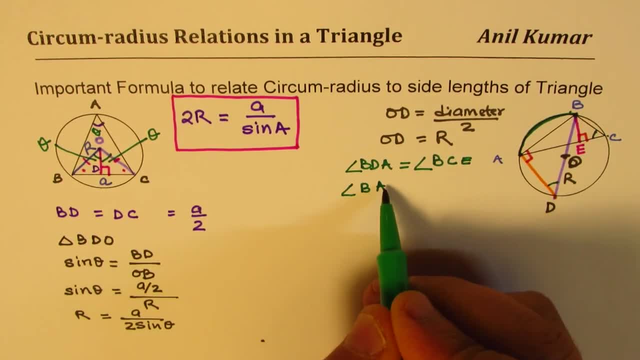 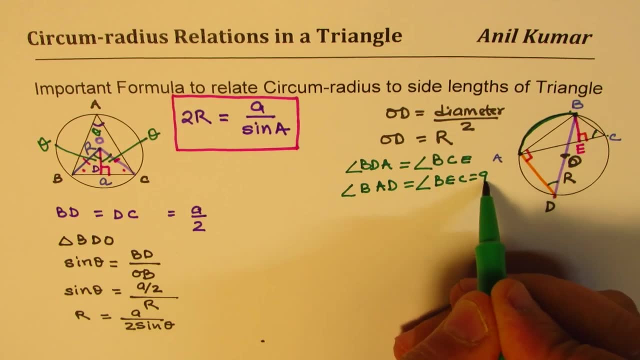 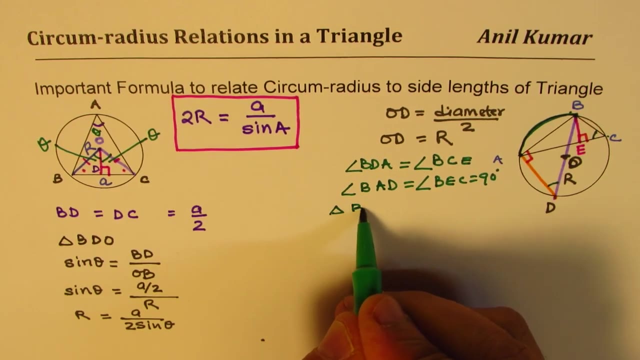 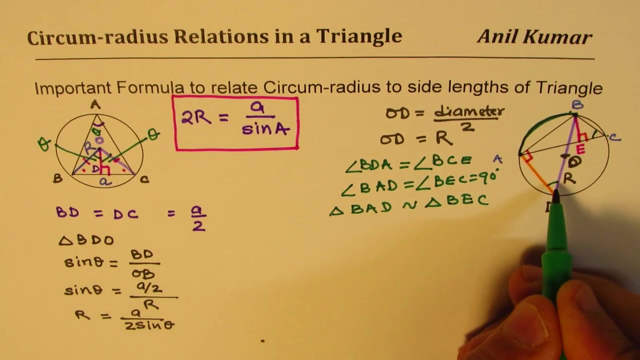 we know angle be a D is equal to angle B. easy, both of them are 90 degrees. so from this we can say, bisschen Vee, that the triangle BAD is similar to the triangle BEC. correct AA property right, So from. 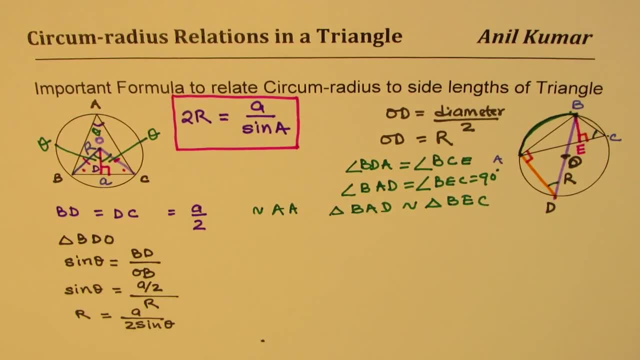 AA property. Is that clear? So these two triangles are similar. Now, once this big triangle and that small triangle, we show that they are similar, In that case we can now say that their sides are in fixed ratio, right? So what we have here is B2D over B2A is basically. 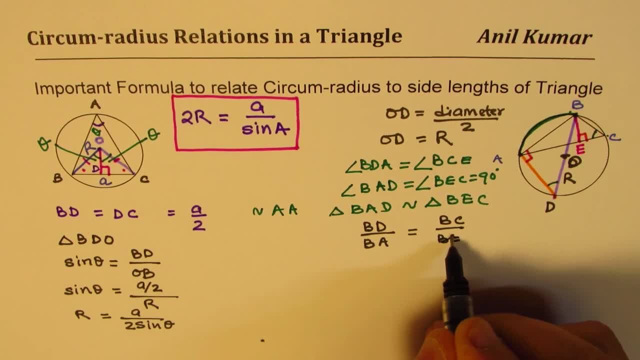 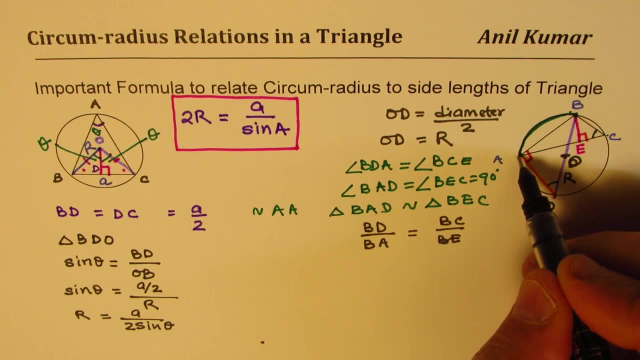 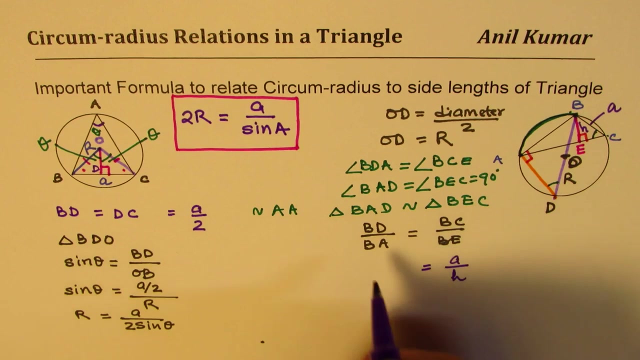 equal to B2C over B2E. right Now B2C is side opposite to A. I will call this as lowercase A, right. So this side I will call as A and this I will call as height. Is that okay? So we could write B2C as A, B2E as H. Now BD: B2D is 2 times R and B2A. 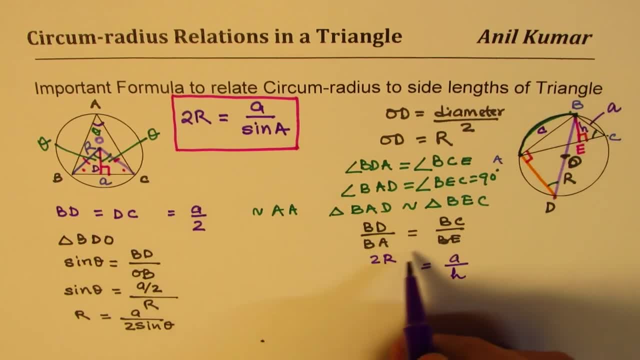 this side is opposite C, So we will name this as C. Is that okay? So this will be side C. So we just name them as per our triangle sides. Now this height H, we can relate with the area of the triangle, correct? So for the triangle ABC. 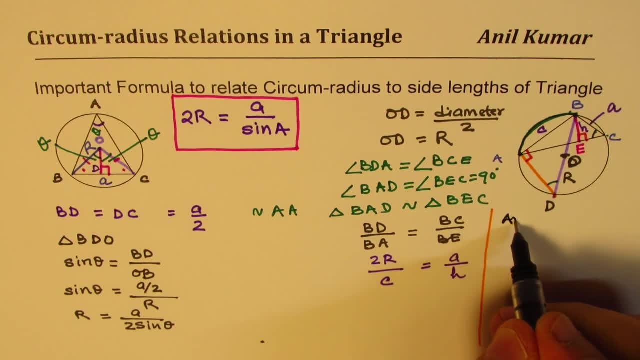 what is the area of triangle ABC? The area A is half of base AC, which is B times height H. So from here I can write that height is 2A divided by B. is height Now replacing that? 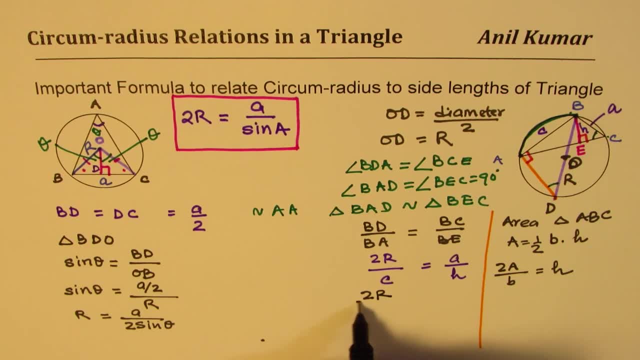 height. in this formula. what do we get? We get 2R over C equals to A over instead of height. I am writing twice area over B, correct? Now we can actually correlate the radius with the area of a triangle and the sides of the triangle. So if I cross multiply, take C on this. 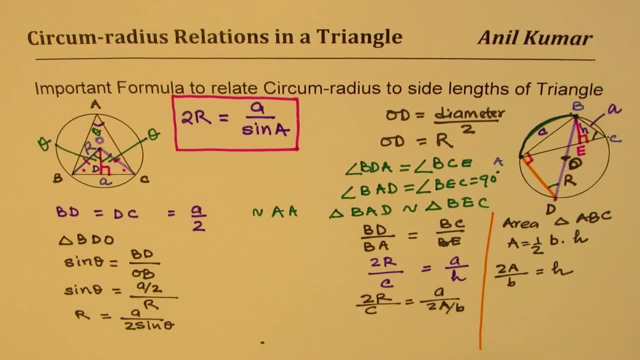 side that B comes on the top. we get ABC in the numerator and this 2 in the denominator. So we can write: R is equals to ABC over 4A. Is that clear? So we cross multiply to isolate R. 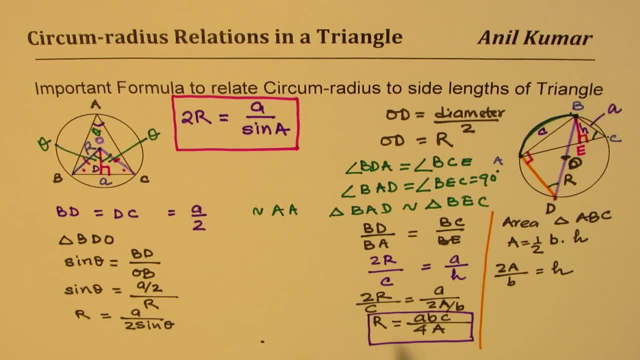 Does it make sense to you? So R is ABC divided by 4A. So if we know the area of the triangle, in that case we can find the value of circumcenter radius using this formula, correct. So that is a very good way of relating them. So that is the second formula.